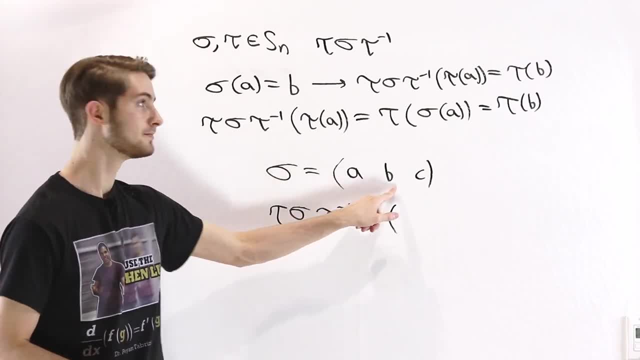 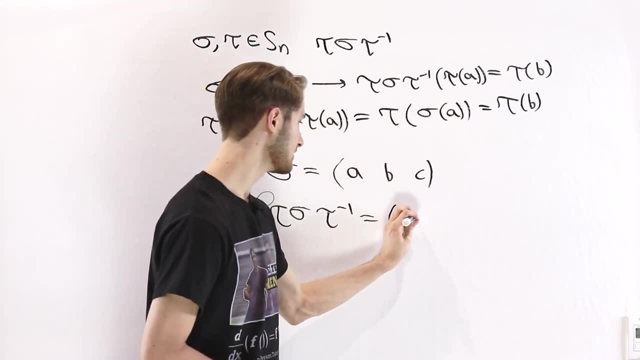 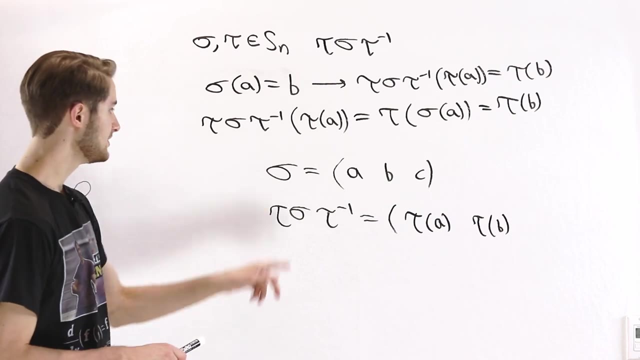 Well, we know sigma is sending a to b, so sigma of a equals b. We know that that means for the conjugation, tau of a, that's going to be the first element of our cycle, and that's going to go to tau of b. Similarly, we see that sigma of b is equal to c. 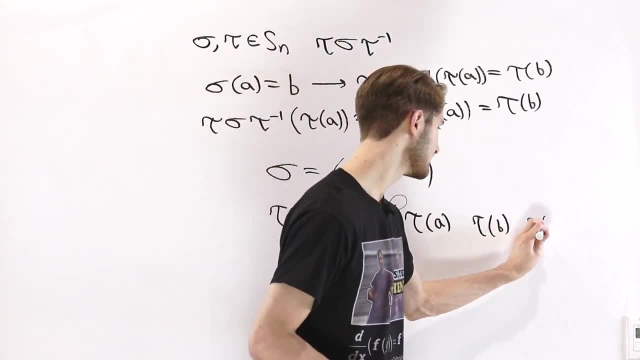 So, as soon as sigma of b equals b, then remember that sigma c is the second element of our cycle. Silver circle is going to beerto the forward what we've been lost in. 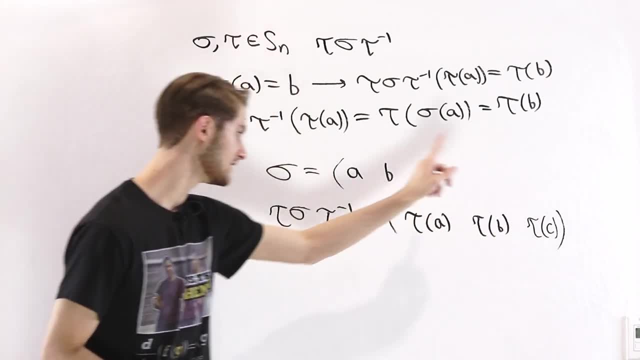 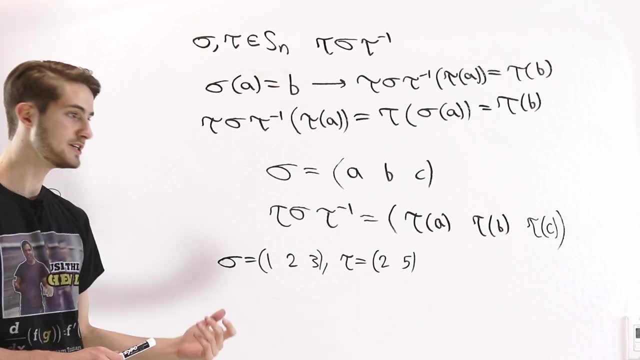 To get our final term of this equation, we are going to use these two operators, so to a, and to b, we are going to take national Marines and give them equal quantities of sigma tau of c. Therefore, this applies to tau of b is going to give us tau of c. 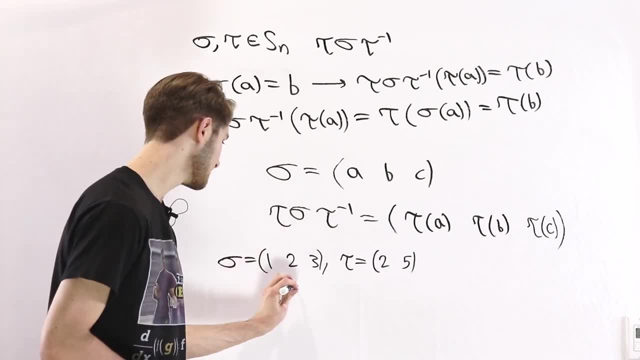 And that finishes our cycle because sigma of c equals a, therefore, this is going to send tau of c to tau of a. icles. 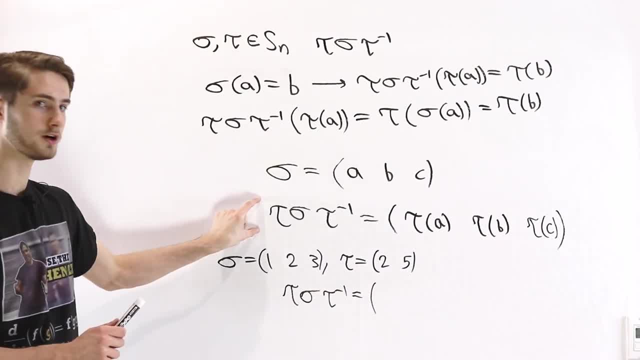 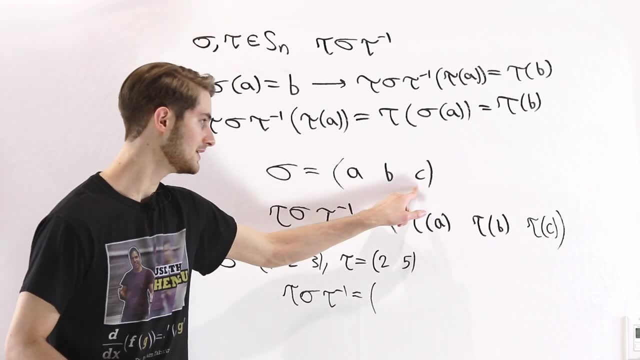 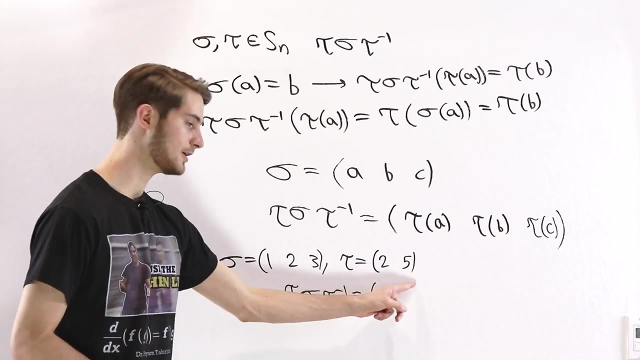 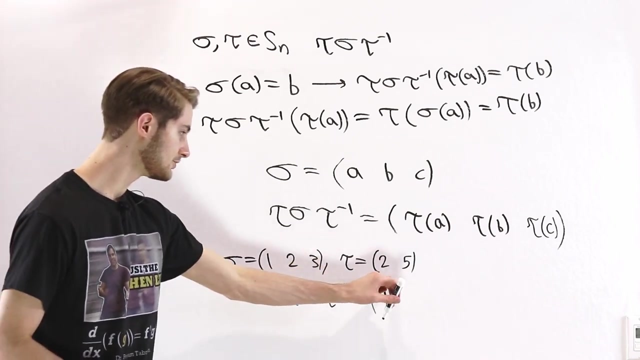 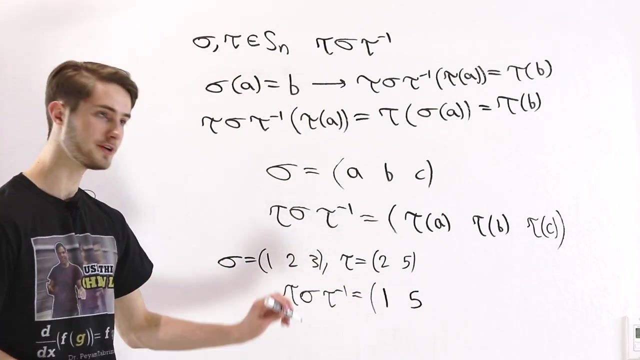 In order to get from sigma to the conjugation, all we have to do is take the elements inside of this cycle and replace a with tau , b with tau , and c with tau . So in this case, 1 is going to get sent to tau , while tau doesn't permute 1 at all, so we're still going to have 1 as the first element here. If we look at 2, tau is equal to 5, so instead of going 1, 2, we're going to go 1, 5. And then tau doesn't move 3 at all, so that's going to be our third element still.